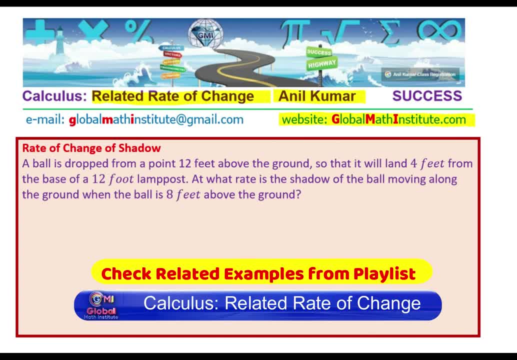 The question here is: a ball is dropped from a point 12 feet above the ground so that it will land 4 feet from the base of a 12-foot lamp post. At what rate is the shadow of the ball moving along the ground when the ball is 8 feet above the ground? So this is an application question. 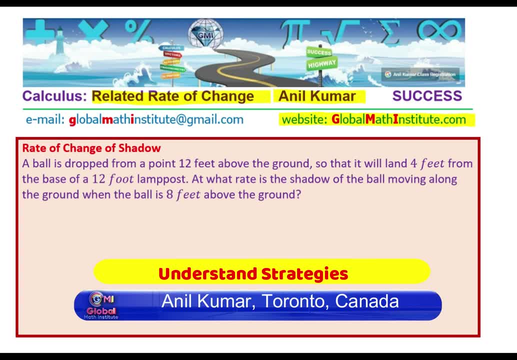 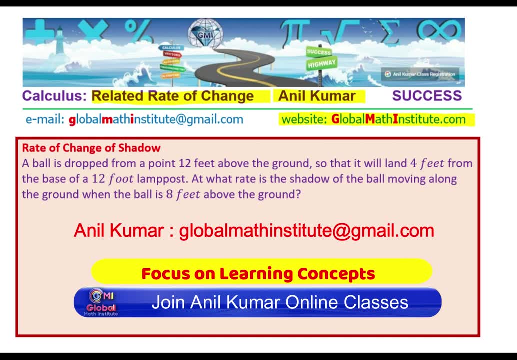 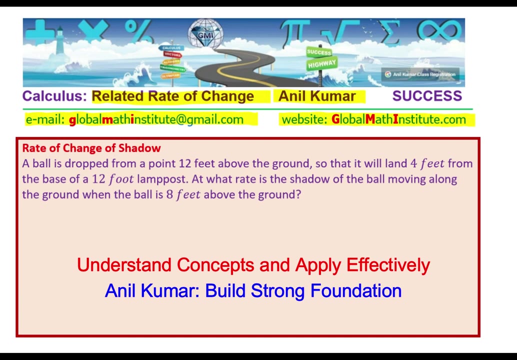 for which, first, you need to write down the equation and then solve it. Well, in case you want to learn from me, feel free to send an email on globalmathinstitutecom at gmailcom. Now let's look into the situation and understand first, and then we'll get into its. 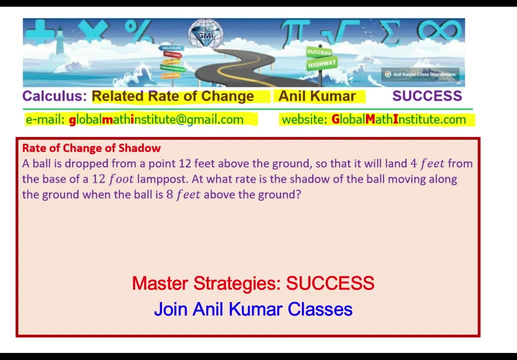 solution. So let's say that's the ground and a ball is being dropped along this line and it falls 4 feet from a from the base of 12 feet lamp post. So let's say that's the ground and a ball, so let the lamp post be right there. Okay, so it falls 4 feet, so that is 4 feet Now as the ball. 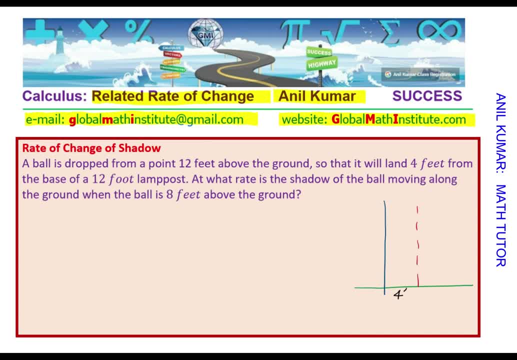 falls, there will be a shadow on the ground. Let us represent this shadow where, let's say, this is the light on the top of the lamp post and at any given instance of time. Let me write down the shadow length. then we see also that the shadow length is off. Well, in the case where the ball is, 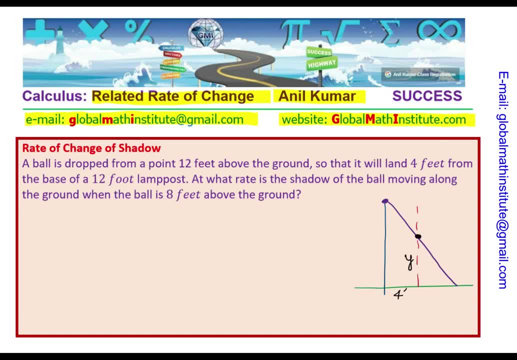 belonging to this new ball. this is just another go. We see, once the shadow length falls, let's simply multiply it with the shadow length and draw a better line here. The situation will be kind of like this: if the ball is that height of Y, for example, In that case shadow length will be X. So that becomes the shadow length. we are interested in finding the rate of change of shadow length as the ball is falling. So you see the length is decreasing most of the Looking at a table model, we see 18 adaptiveachtechnology, which isある, and this is aplicability for this graph. 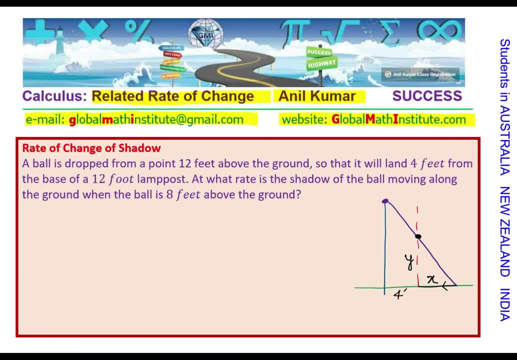 But as a group we see 11 magnets somewhere, For the same that we form 10 magnets around the survive between the lambda. but this is just applying 2 the type, so you expect a negative answer. perfect, we are also given that this lamp was just 12 feet. 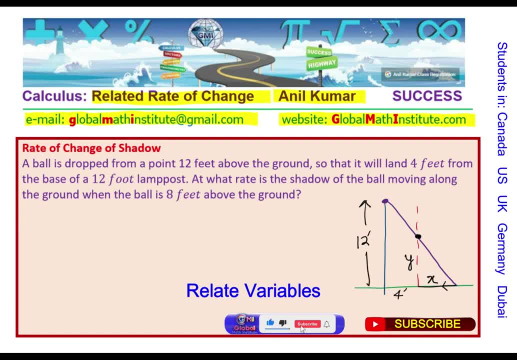 high and ball is also dropped from the same height, correct? so how do we relate x with the height y? that is what you need to figure out. so in phoenix we have learned that the height can be written as initial height 12, right, in this case, let me write h 0. give you a formula. first now, since it's falling, so it is decreasing at the rate of. 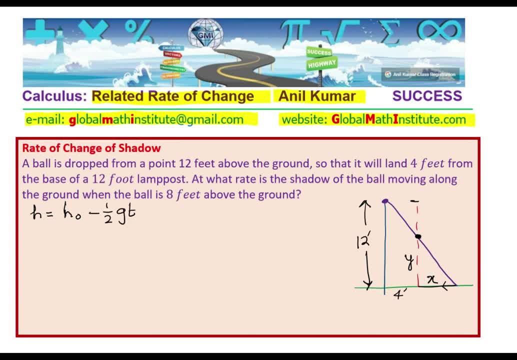 half gt square, where, of course, t is greater than equal to 0 and g, since we are talking about feet, is 32, so we are going to write gt feet per second square. make clear. so that is what your basic equation is. in our case, we are. 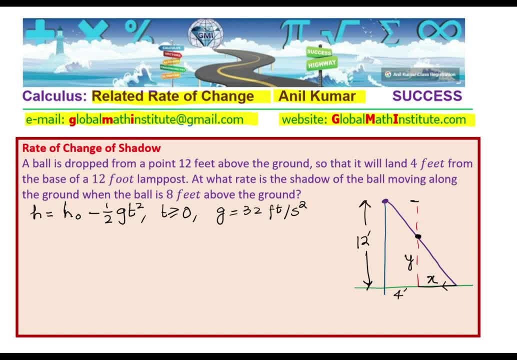 considering height at any instance of time as y, so i could write this as: y equals to, and initial height is 12 minus half, 32. for gravity acceleration: t square, correct. so you can write down the equation simplified form as: x, 12 minus half of 32 being 16 t squared, so that becomes the. 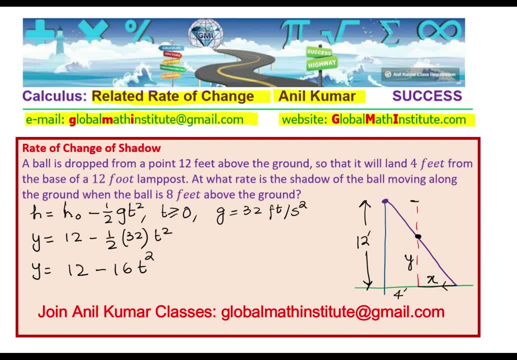 change of height with time. right now, what we are given here is that at what rate is the shadow, the ball, moving along the ground when the ball is eight feet above the ground? so when the ball is, let us say, eight feet above the ground, let's say this height is 8 feet above the ground, when the ball is about 10 feet above jej. 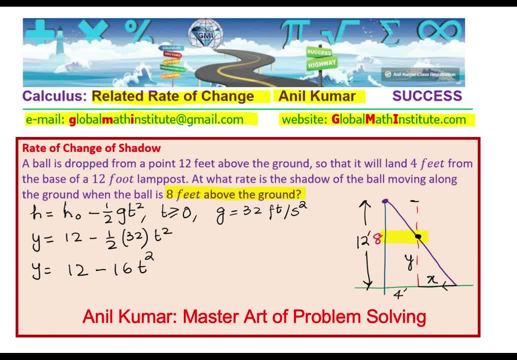 8 feet 5 meter above the ground. let us say this height will not be measured. thousand feet right is 8. so at this instance we need to figure out the rate of change, right? okay, so let's find the instance time right. so if I put 8 as the height, I get 12 minus. 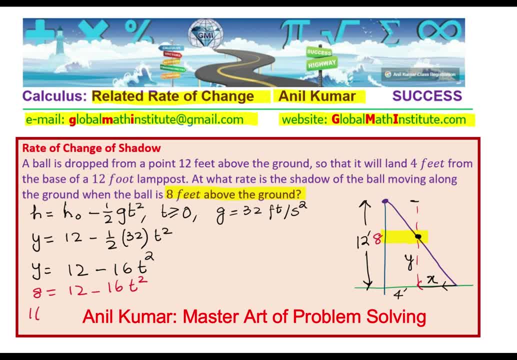 16 T square. 16 T square equals to 12 minus 8, which is 4. and now we can solve for T, which is T square, equals to 4 over 16, which is 1 over 4. so T will be equal to square root of 1 over 4, which is half second right. so after half second, the 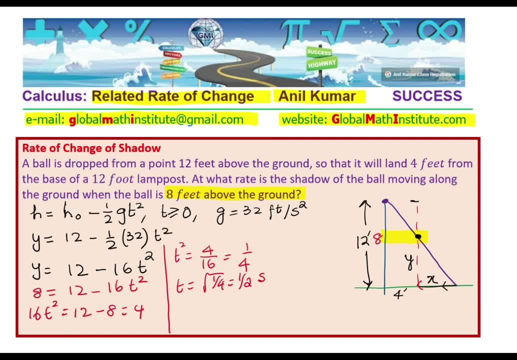 height of the ball is 1 over 4, and the height of the ball is 1 over 4 and the going to be 8 feet. is that clear to you, right? so we got the time now. so we know that T equals to 0.5 or half seconds at this time. perfect. so lot more things to. 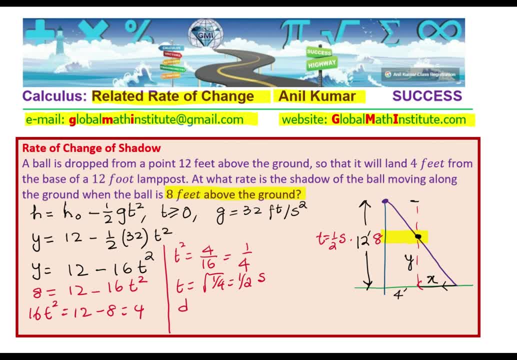 be done now. we need to find what is DX DT when T is equal to half second. is that clear to you? this is what we need to figure out, so I hope this situation is absolute. be clear, so we'll move forward and then solve it. relating X and Y to find DX DT. 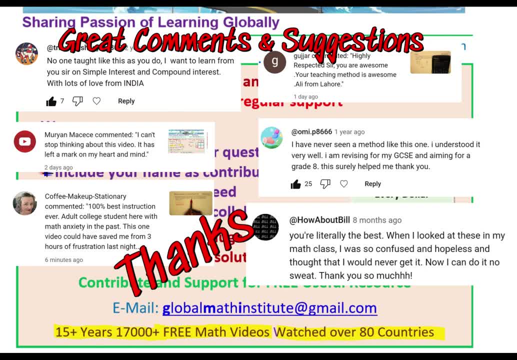 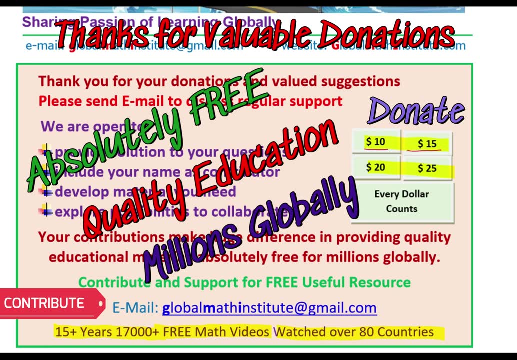 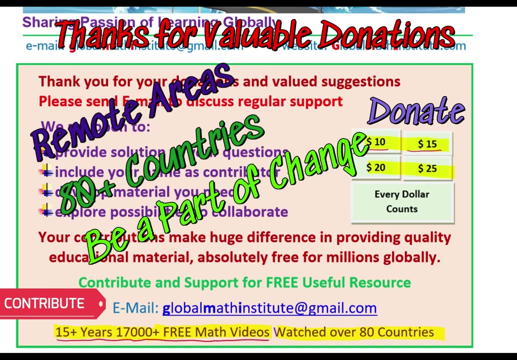 meanwhile, let me thank all the subscribers and viewers who have been watching my videos, posting excellent comments and suggestions. special thanks to those who are providing us with some contributions to sustain growth. we have been serving you for last 15 years absolutely free, with 17,000 videos now which are being washed over 80 countries. 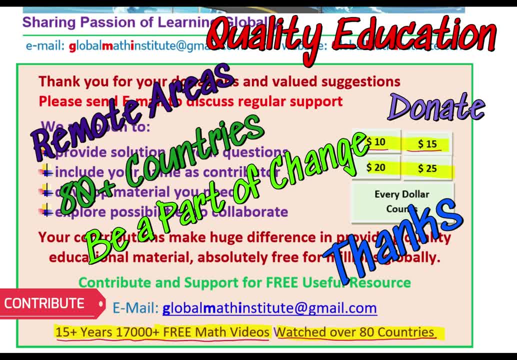 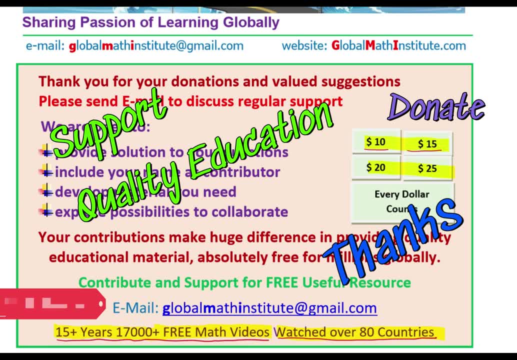 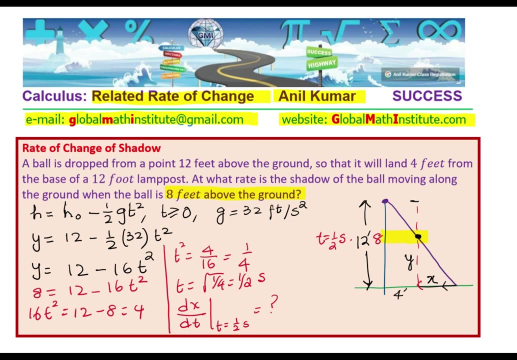 most important thing is the quality which we provide. access to this quality in remote areas is something which we want. that's our passion, and your support can help us reach millions globally. so keep supporting, thank you. so let's get back to the solution. so so we figure out that in this situation, time will be half second when the 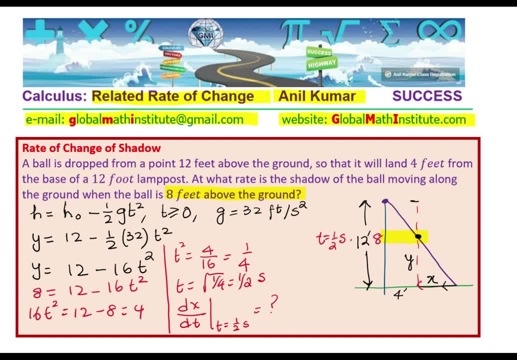 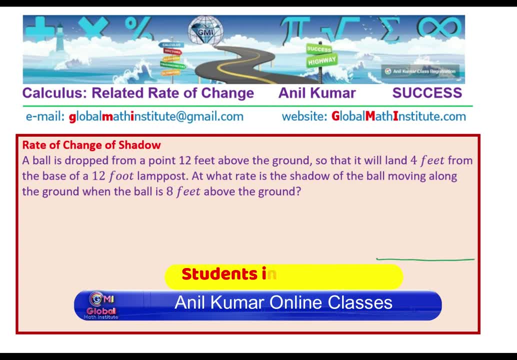 ball will be 8 feet above the ground. so on the next page, let us now see how do we further solve. so let me repeat here, sketch the diagram which we just made and, as you can see, the focus now is to relate X and Y, y being the height and x being the length of the shadow where the ball is falling four feet. 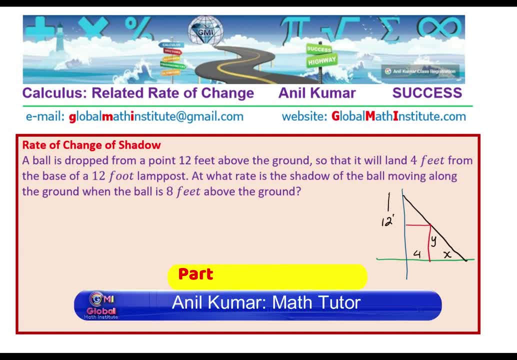 from the post, which is 12 feet high, correct? so? so we can now relate, if you see a small triangle and the big triangle, which is similar triangles, right, so? so this small triangle is similar to the big triangle. in the big triangle, height is 12 and 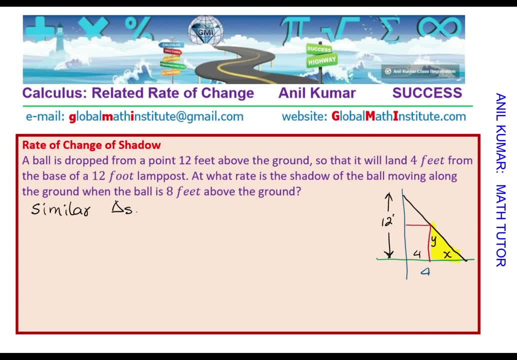 the point base is 4 plus X. so from similar triangles we can relate this to. X over Y is equal to 4 plus x over 12. Make sense. So that becomes the relation and we can relate x and y. We have already figured out that y is equal to in the last page. y is equal to: 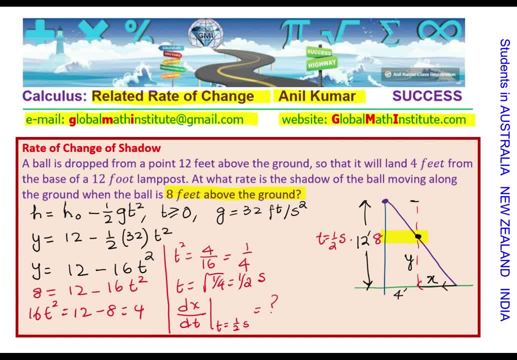 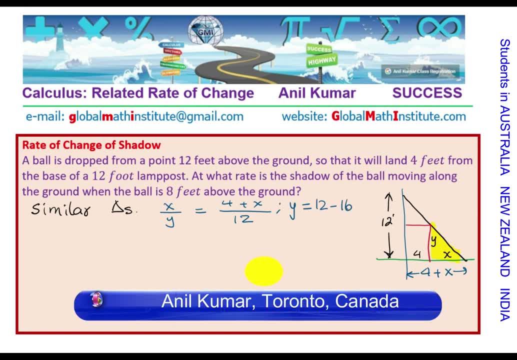 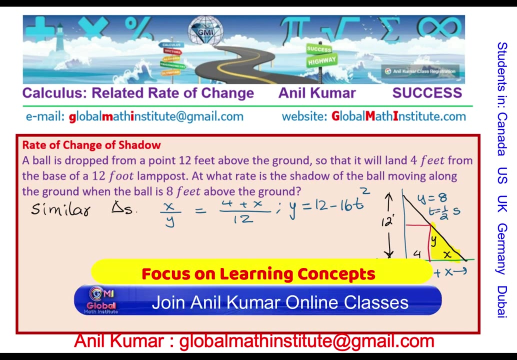 12 minus 16 t, square right. We also found that at when y equals to 8, t equals to half seconds, right? Okay, great. So we have all this. Now let us isolate x, right, So? what we are doing is we are taking the y-axis right. We are taking y-axis right And what we have found is that when t equals to 12 minus 16, t square right. So we are taking the y-axis. 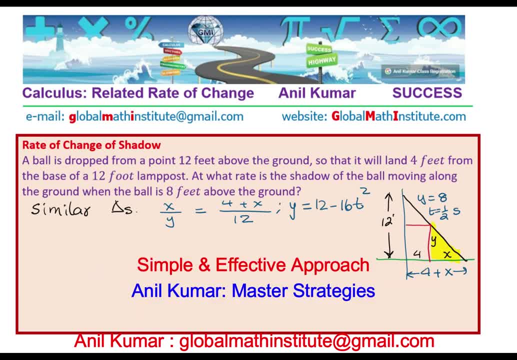 going to do is take y on the other side, or we can just cross multiply first. so let's do this part. so we get 12x equals to 4y plus xy. so I just cross multiply now, bringing X together, isolate X by taking it as a common factor. so X. 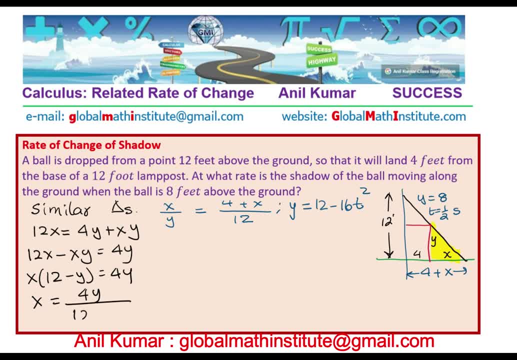 is equal to 4y over 12 minus. very clear. so we have an equation where X is 4 y over 12 minus will clear. now let's find the rate of change. so dx, dt is equal to apply the equation rule. so derivative of 4y will be 4 times y prime minus. 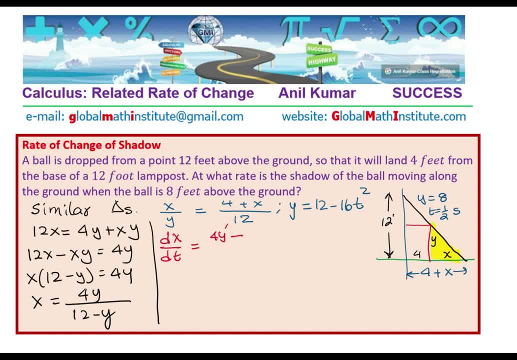 derivative times. sorry times, 12 minus y. question rule: right minus derivative of denominator, which is minus 1 times 4y and minus 1 y prime right divided by. we are differentiating with respect to time t. OK, So this is when we differentiate with respect to. 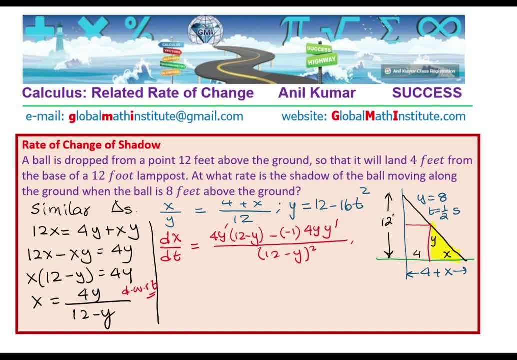 time t. So that is what we get. We can now simplify this a bit. y prime, as you can see, is common right, So we will take y prime here And 4 times 12 minus. so we will open the bracket. 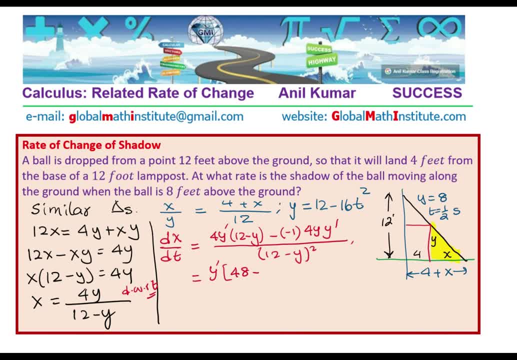 4. times 12 is 48 minus 4 y, and this is plus 4 y over 12 minus y. whole square clear. Now we need to find what is y prime, right? ok, Let me simplify it further. So we have. 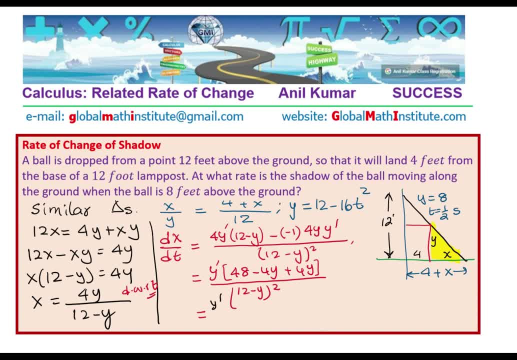 let me change the equal So y prime times 48, because minus 4 y and plus 4 y will cancel. so 5 prime times 48.. Over 12 minus y, whole square, correct. So we have got the expression for the derivative. 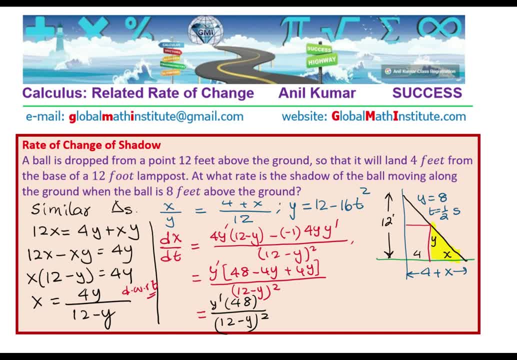 correct, which is dx, dt. You need to find what is y prime at. t equals to half second when y equals to 8.. So we know all of the values. x is given to you as 4, right? So the only thing which you want to find is y prime. So let us take it on a new page. 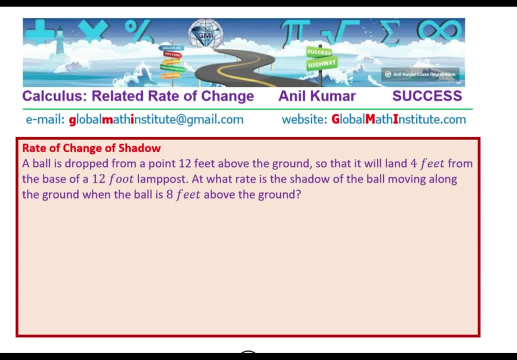 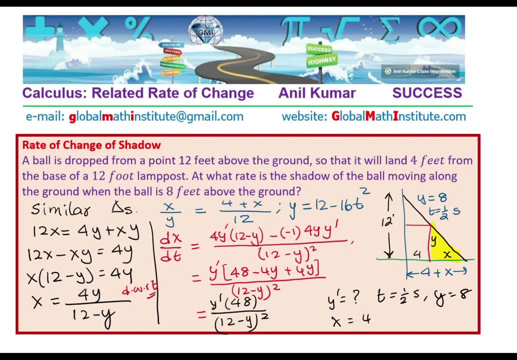 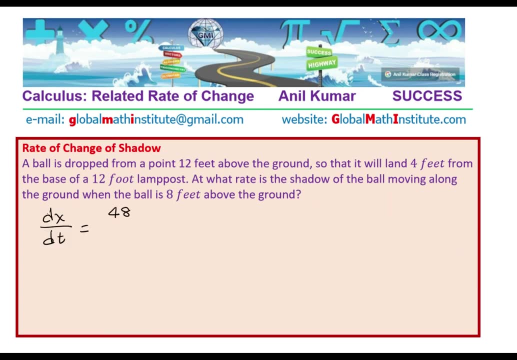 We will just figure this out. So dx dt is equal to: we have 48 y prime over y minus 12, sorry, 12 minus y whole square. Ok, So we also found that the equation for the height y was 12 minus half gt square, so 16t. 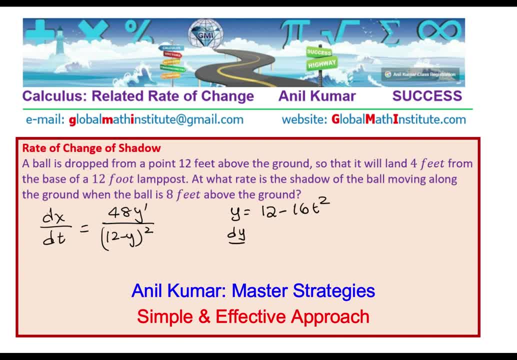 square. So from here we can find the derivative: dy dt will be minus 32t right Now, since we know t equals to half. so we can say: dy dt for t equals to half is well. So minus 32 times half, which is equal to minus 16, so we have y prime now, correct? 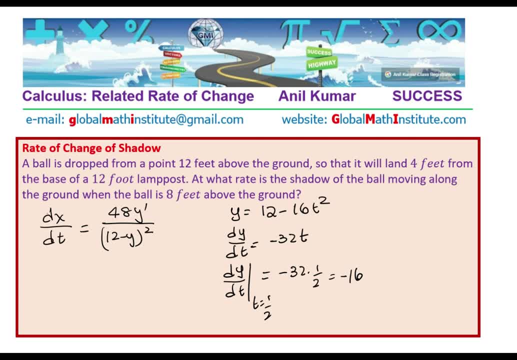 So we can say that dx dt equals to 48 times minus 16, right, and this is when t is equal to half. So when the height is 8, right, and we have 12 minus 8 whole square, correct. 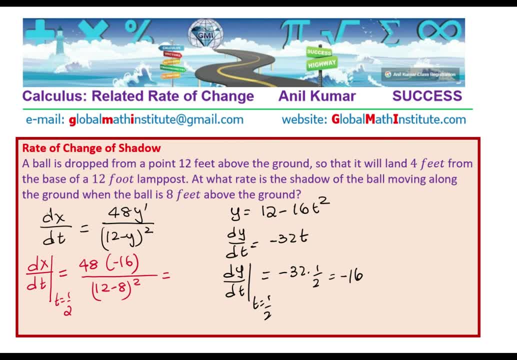 So 12 minus 8, whole square is 16, so we have 48 times minus 16. over 12 minus 8, 4 square is also 16.. And when you divide, what you get is minus 16.. So we have 48 times minus 16. over 12 minus 8, 4 square is also 16.. 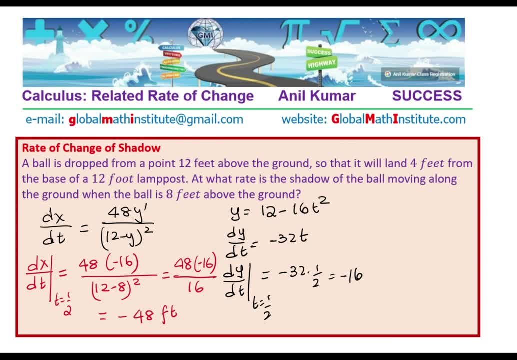 And when you divide, what you get is minus 16.. So you get minus 48 feet per second square. Is that clear to you? So that is how we are going to calculate this particular value and that is the answer. ok. 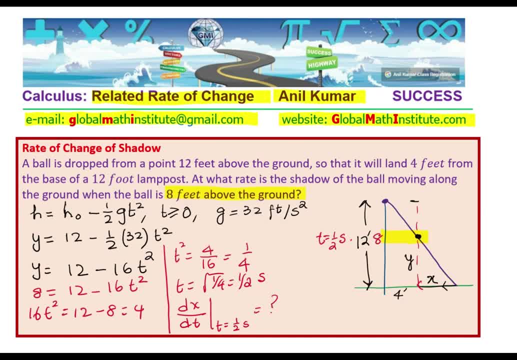 So now let us look into the steps which we follow. We begin by sketching the diagram ball being 4 feet away from the lamp post, which is 12 feet high. So the height of the ball is given by 12 minus half 32 t square right. 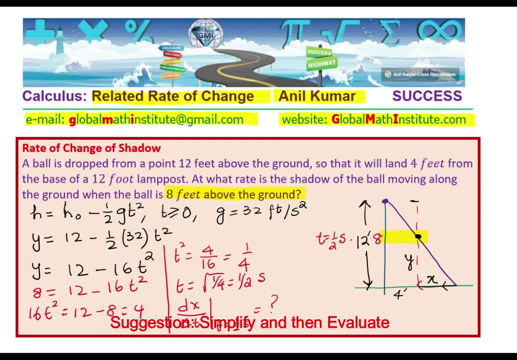 So this is a 12 foot diameter lamp post which is 12 feet high, And this is also 12 feet. So the height of the ball is given by 12 minus half 12t square plus gt squared. right simplified this to minus 16 t squared When y was 8, t was half seconds. So we have 8 and 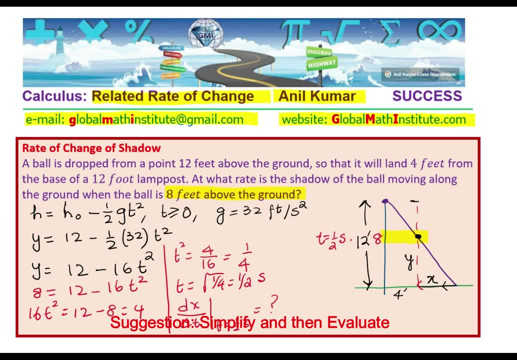 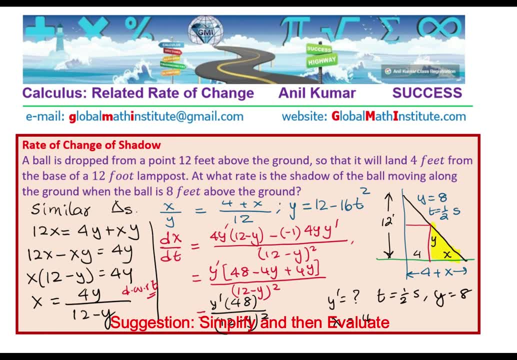 half seconds right there And the equation is: y equals to 12 minus 16 t squared. Then we related the two similar triangles x over y with 4 plus x over 12, cross, multiply and solve the equation So 12x, bringing x together on the left hand side and taking it. 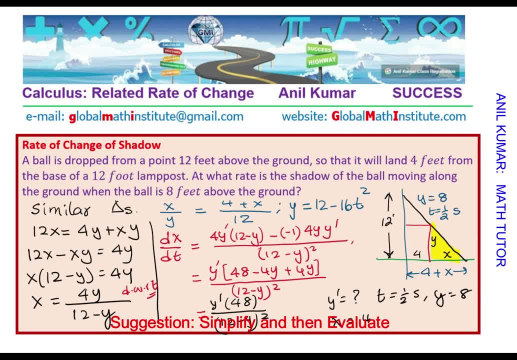 common. we got 4y divided by 12 minus y is x. Now differentiating with respect to time, applying the quotient rule, we get the derivative as 4 prime times 12 minus y, minus derivative of denominator, which is minus 1 y prime times 4y. 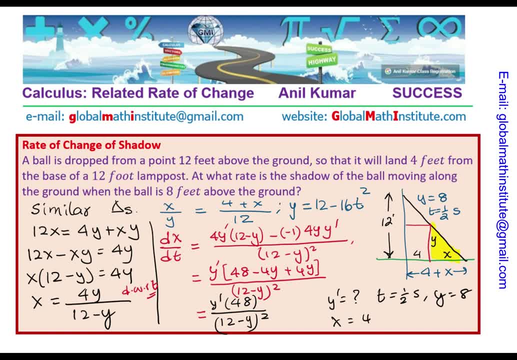 So we took y prime as a common factor and multiplied 4 with 12, giving 48 and minus 4y. with y, added 4y correct 4 by 4y, cancel giving us 48 y prime over 12 minus. 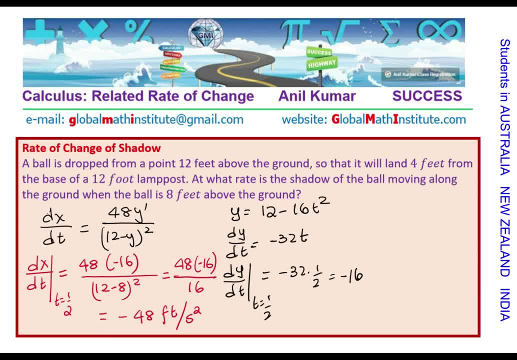 y whole square. So that was our equation. And finally, to find the y prime, we differentiated the equation: 12 minus 16, t squared, getting minus 32 t. Substituting t as half, we got minus 16 and then placed minus 16.